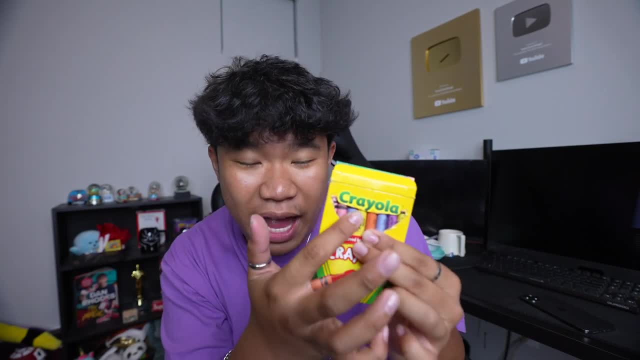 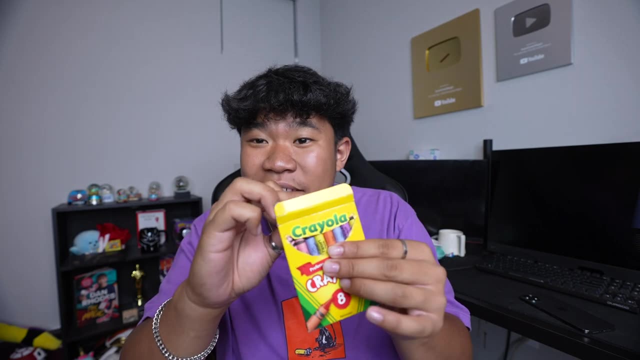 What you want to do is place it inside of the box. now some boxes will have this opening where you can see the crayons. If your box does not have an opening, just cut one open and bam, You should be able to see it. To be able to see the crayons when they are at the top half of the box. 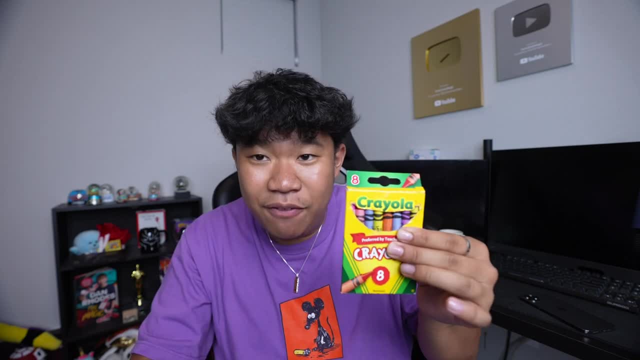 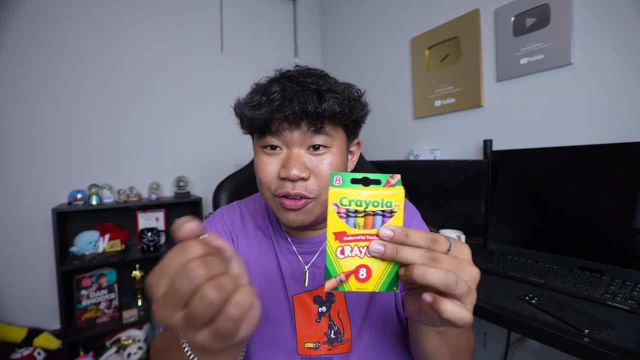 And that's all you need to set up. have the crayon sticking up at the top half, and to make them vanish, All you have to do is wave your hand over and drop The crayons down to the bottom. when you do it all together, to look something like this: and the crayons are now vanished: boom. 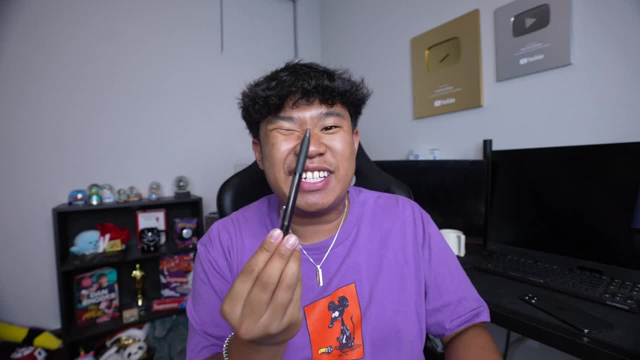 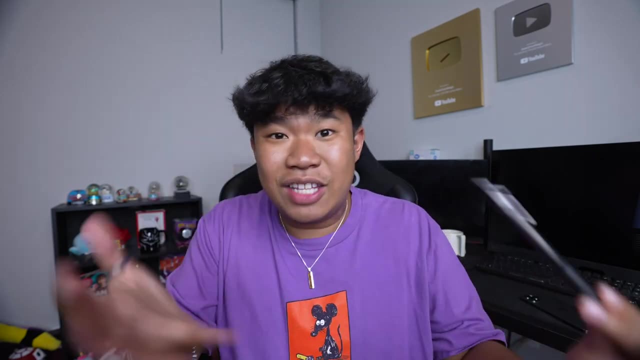 Instant magician. the second back-to-school magic trick that I'm gonna be teaching you all today is how to take any pen, Stick it up your nose and out your mouth. Oh, this magic trick has got to be one of my all-time favorite magic. It's not one that I just do at school. 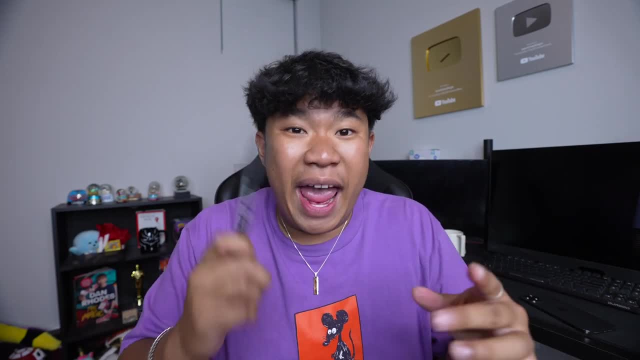 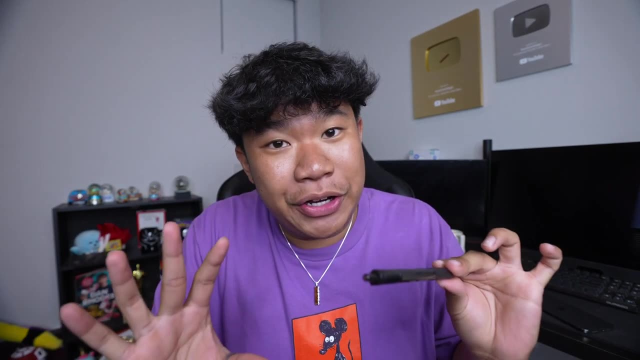 It's one that I do everywhere that I go, whenever I'm performing or any occasion where there might be a pen on the table, I just go, Like that catches people really off-guard and it's pretty simple to do. So what's happening here is you're not actually shoving the pen up your nose. 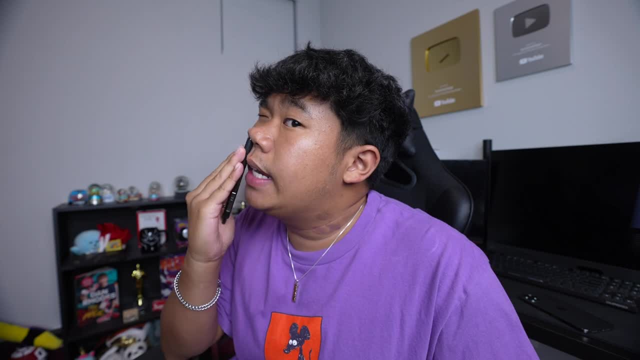 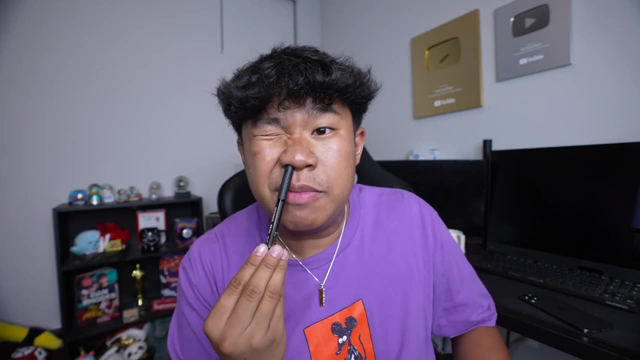 What's happening is from the back. The pen is actually gliding the side of your hand like so, and you're using your teeth To pull it out like that. when you do it all together, It should look something like this up: the pen is right there and 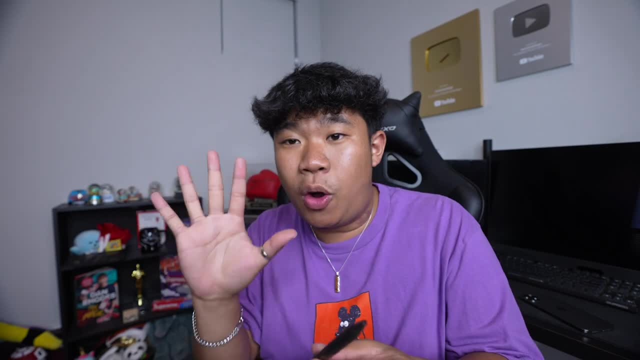 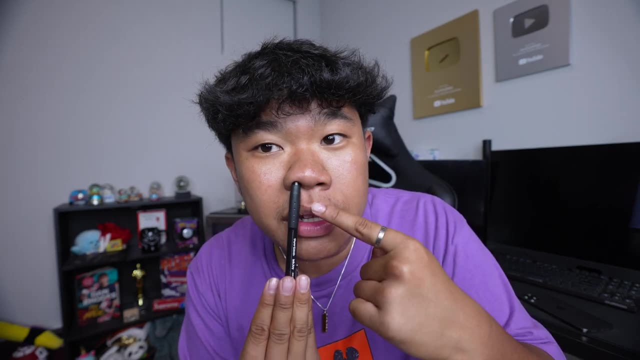 Then down the pen cutter comes out. So let me break this down. how you want to hold is you want to hold The four fingers on the front of the pen, thumb in the back, and what you're gonna do is you're gonna press This pen to the top of your nose and no, you're not actually gonna push it in. don't do that. 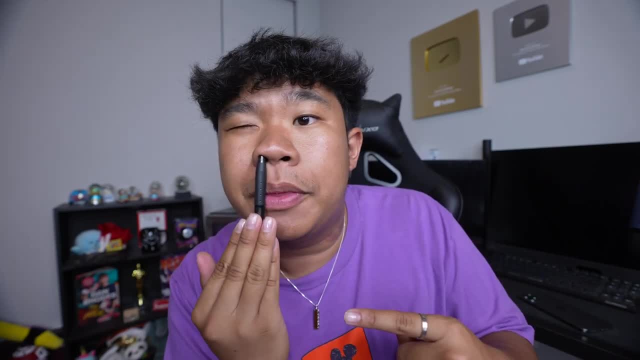 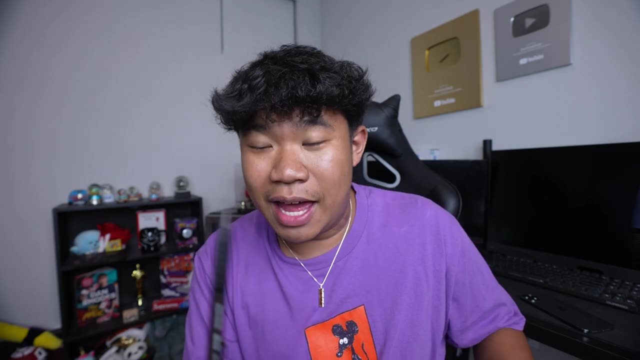 Be very careful, and what you're gonna do is you're gonna use your hand and glide up the pen, like so, Using your thumb to grab the pen, and then you're gonna grab it with your teeth, Just like that. once again, all together with some practice, It should look something like this: 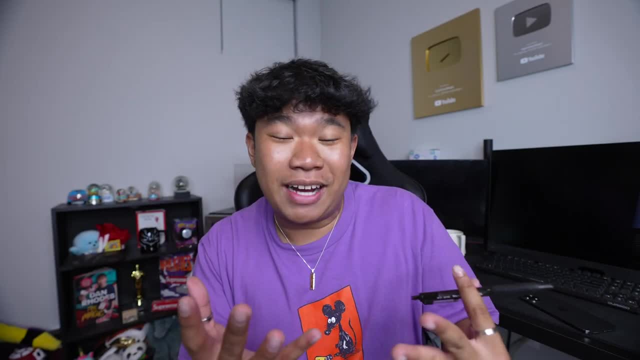 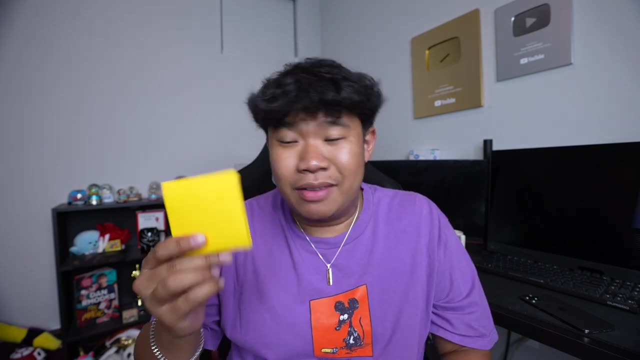 You can add the little sniffing and whatnot Sound effect, and the more practice you get at this, the better It'll look. the next magic trick I have for you uses sticky notes. do kids even use sticky notes these days? Anyways, what I'm gonna do is I'm gonna draw something on the sticky note. all right, as you can see, 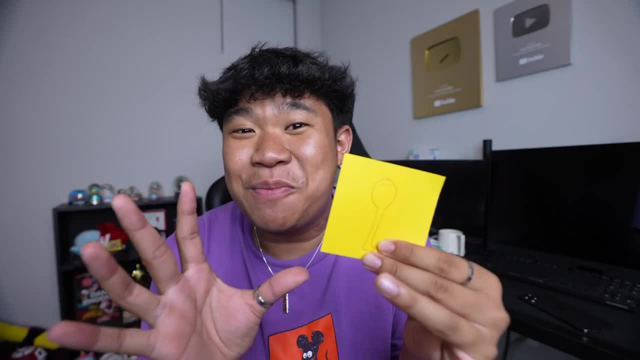 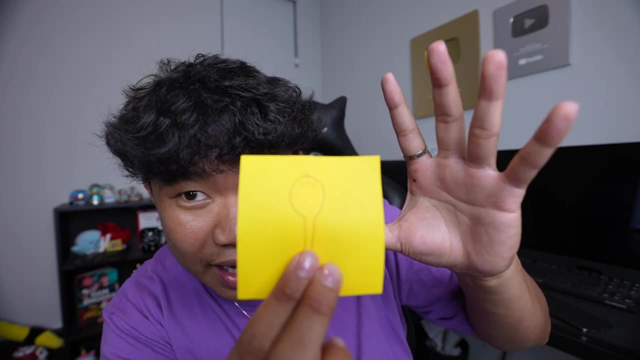 I drew a little spoon on the sticky note and, just like a lot of other magicians who can make spoons bend with their mind, I'm about to do that with this sticky note. if you focus on the sticky note, you notice It actually starts to bend a little bit with the power of your mind. bend a little bit more and a little bit more just. 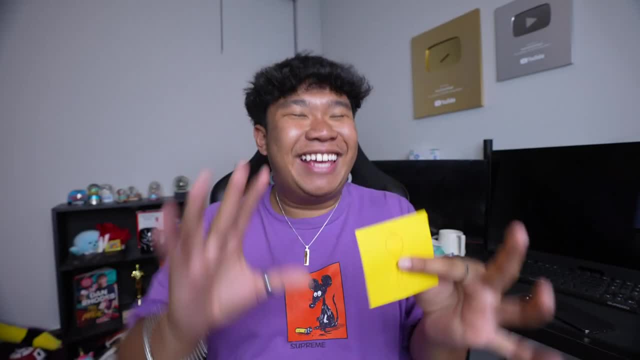 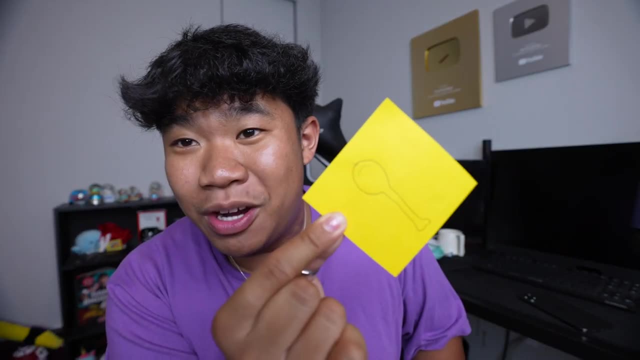 like that. Now, that was pretty cool, But again, like the other, magic tricks, is so, so easy. all you need is a packet of sticky notes and a pen. on one Sticky note, what you want to do is draw a spoon- I'm clearly not an artist, for a reason- and what you want to do is take another sticky note and rip just a little piece. 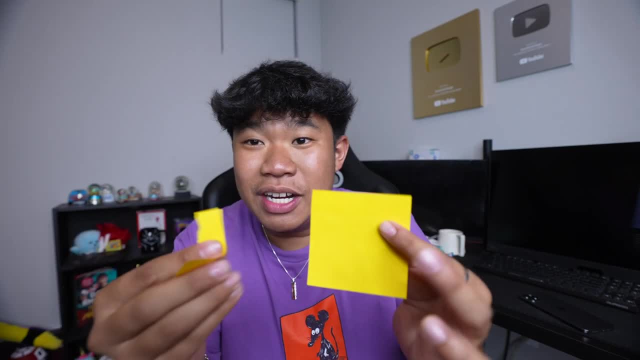 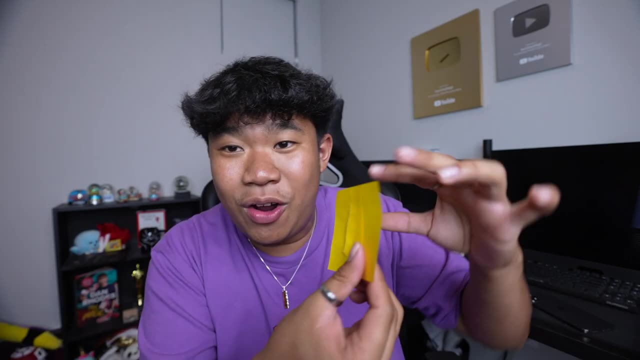 Like: so what you're gonna Do is you're gonna use this piece and you're gonna stick it on the sticky part of the other sticky note, just like so. so Now you should have this little extension to the actual sticky note, and all you're gonna do to do the magic trick is use. 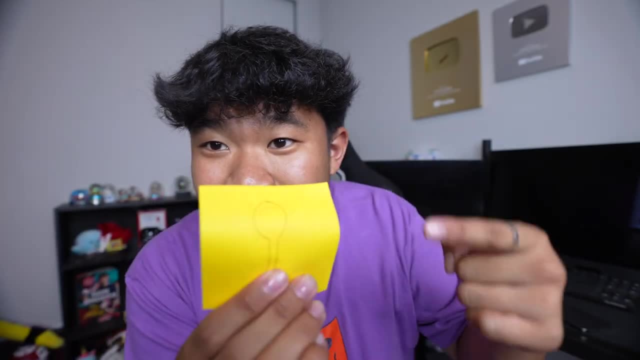 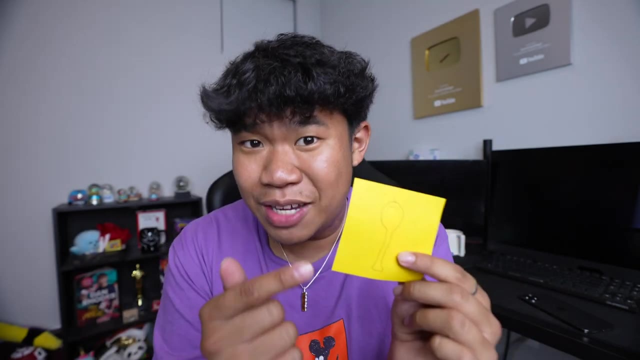 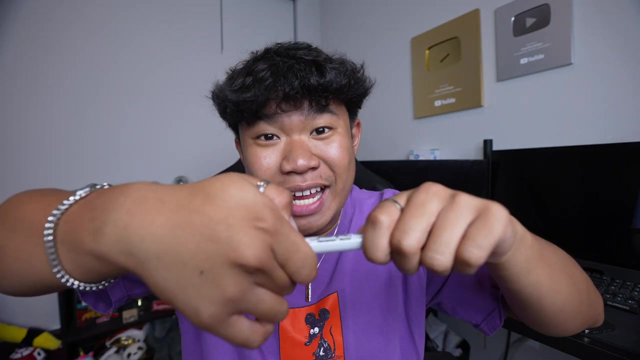 your thumb to pull down the Spoon and it will bring the spoon back, Bending it like magic and, if you want, you can even make it go back to normal, just like that. That's how you bend a sticky note spoon with your mind. The fourth trick that I have for you today is a sharpie magic trick. watch closely with the sharpie if you take the cap off. 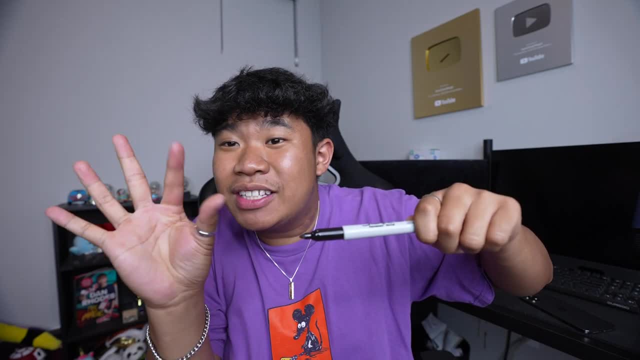 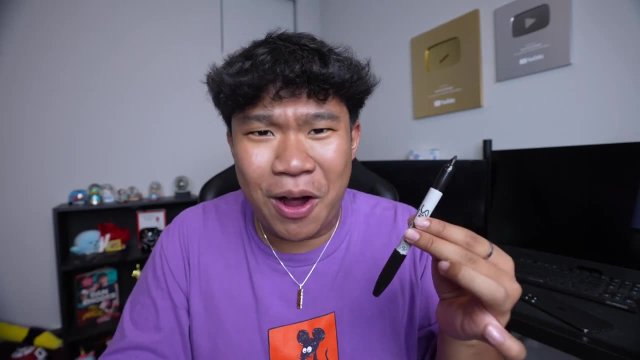 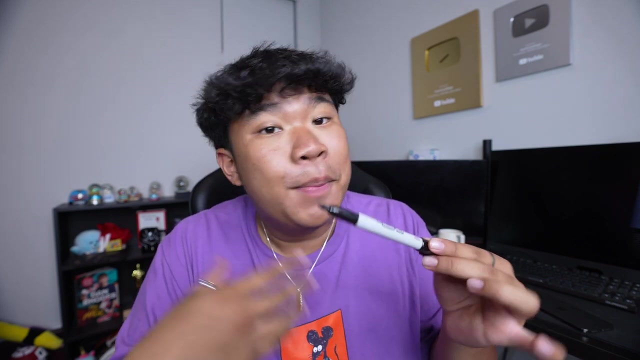 And you rub, You can actually get it to completely vanish, just like that, and then appear on the other side of the sharpie. now, How did I do that? You heard me take the cap off right, or did you? this magic trick plays with your Senses. it makes you think that you hear a cap of a sharpie, but in reality you don't. this is what you're hearing. 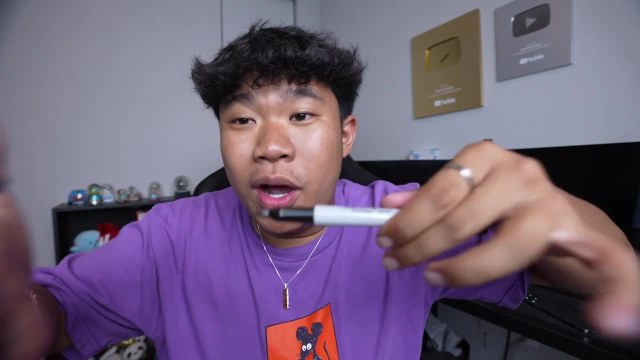 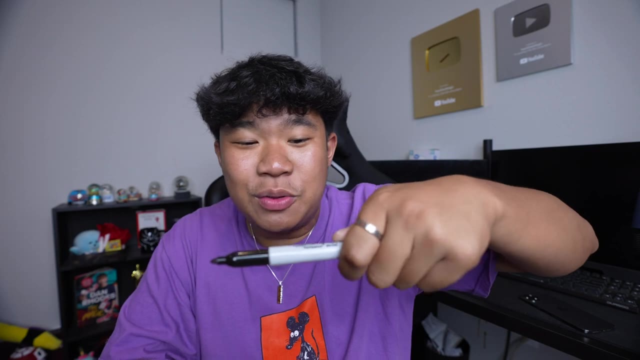 Sounds like I took a cap off, right? nope, No cap at all. what you're doing here is you're messing with their senses. and to start, what you're gonna Do is you're gonna take the cap and place it on the other end, just like so. then what you don't want to do is: 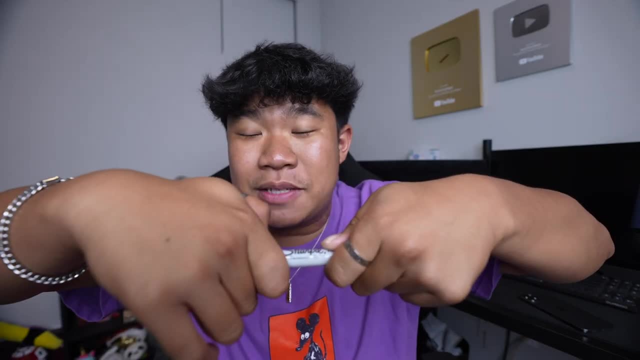 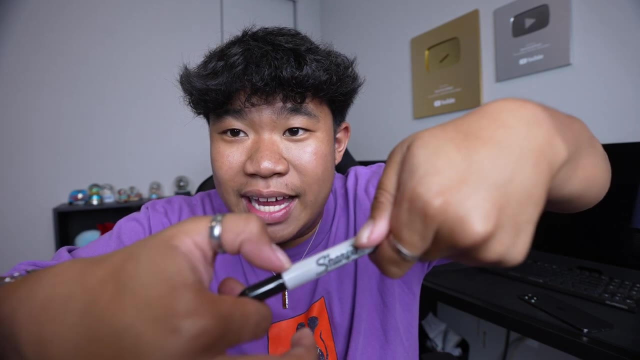 Hold the sharpie covering the cap and then take your other hand and place it on the cap side, Pretending like you're gonna take the cap off and all you're gonna do is you're gonna use your nail, your thumbnail, right here and rub It on this ledge. 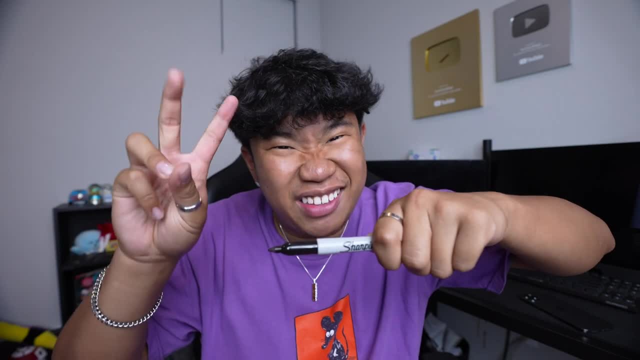 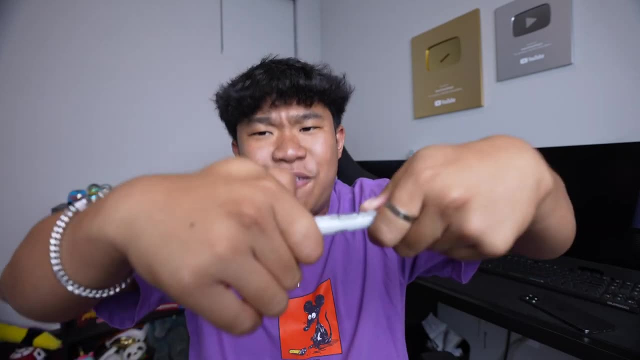 Just like that. when you rub it on the ledge right when you're taking the cap off, it will sound like it's coming off. Just listen, Doesn't that sound like I'm taking off a cap and all you got to do is act? Hey friend, watch the sharpie cap. 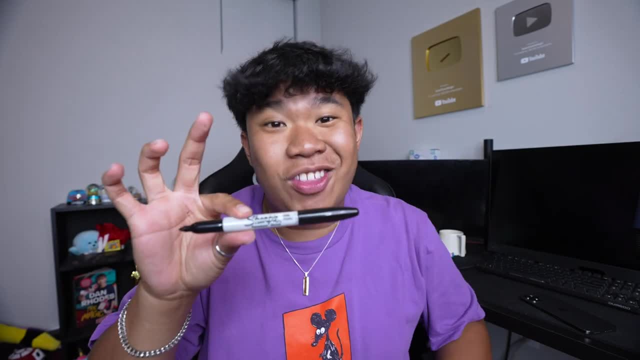 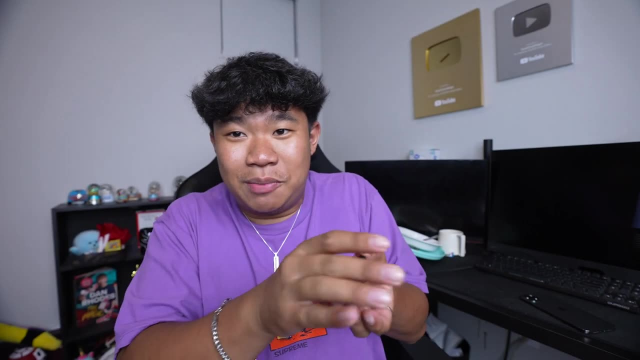 Vanish and it's up in the air and it goes all the way back to the other side. boom, You're an instant teleporter, and the last magic trick that you can do at school also uses the cap. watch closely. It looks something like this: We're gonna take the cap right here and make it completely vanish, just like that. 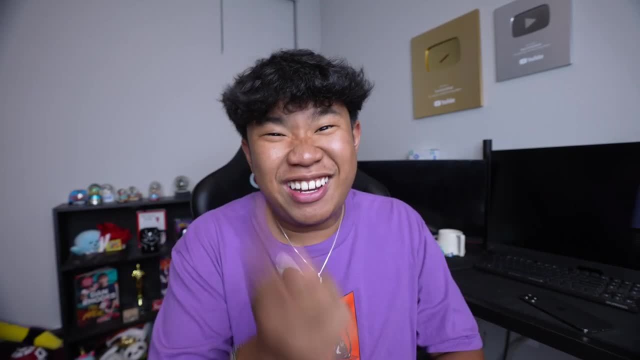 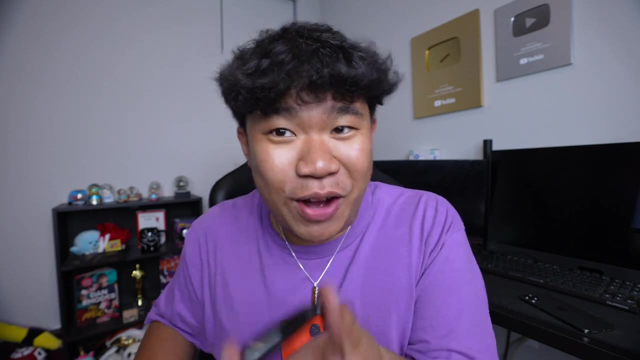 This one is probably the hardest one out of all Of them to do, but with enough practice this will look so good and you can make any small object disappear, Not just the cap. we're gonna be doing this move called the French drop, Which is very common in magic. that looks something like this: 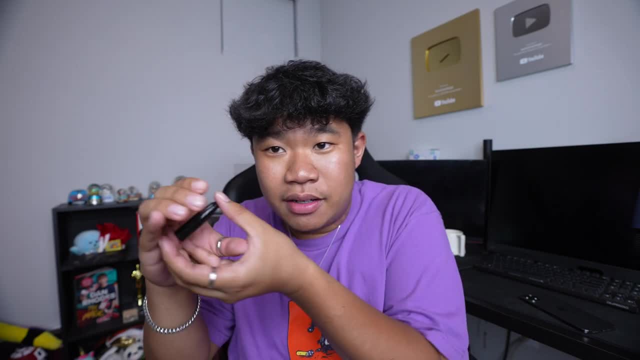 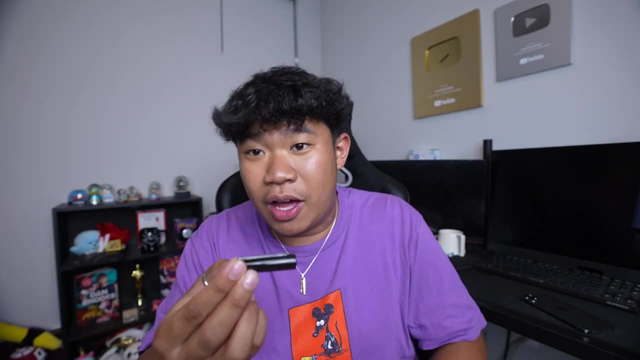 Basically, the move is that while you're covering the front, you drop The small item, in this case a cap, pretend to grab it and then making it vanish while the cap is in the other hand, When you do it smoothly, it looks something like this. So let me break it down. 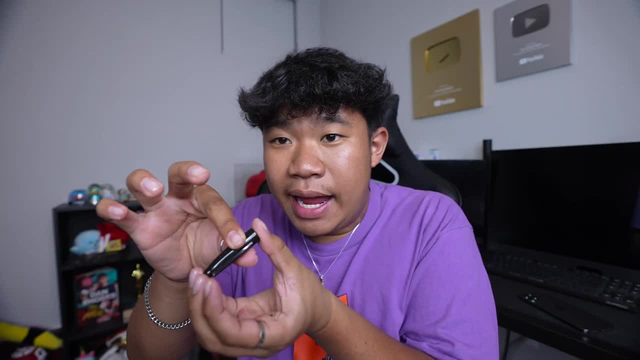 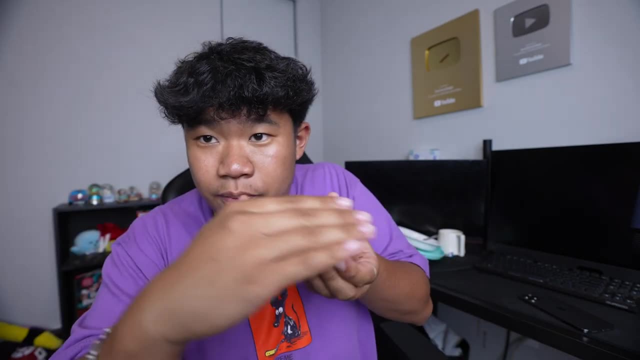 What you're gonna do is you're gonna hold the cap with your thumb, your four other fingers and the other side. this is gonna be your French drop position. and what you're gonna do is you're gonna use your other hand to cover- right cover- but what you also want to do is not have your thumb out, like so. 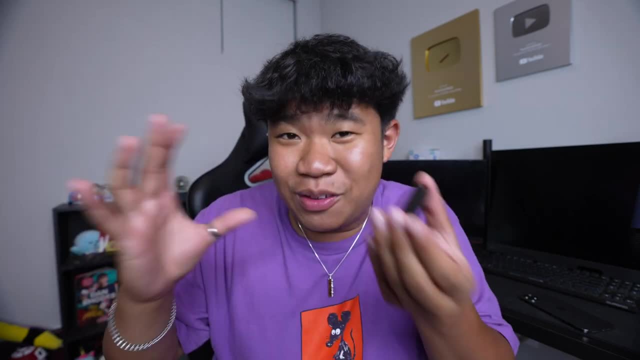 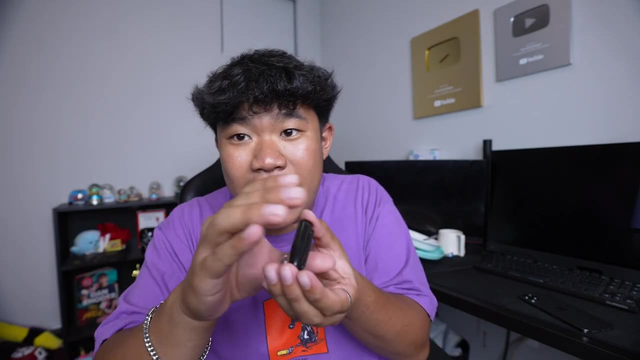 you're gonna have it through this hole. this is a really big key in the French drop and a lot of people practice this. they don't do this right. you're gonna cover, but you're also gonna put this thumb through this hole, like you're actually gonna grab the item right but in reality you're not grabbing it. you're. 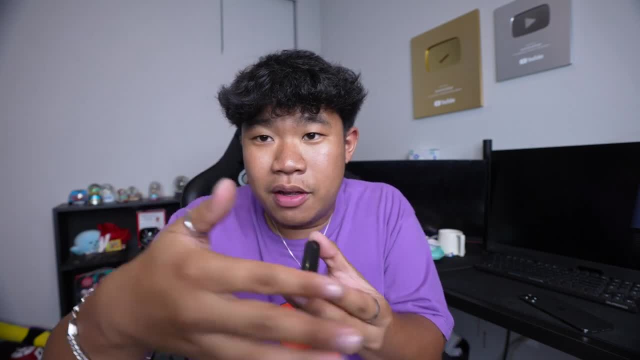 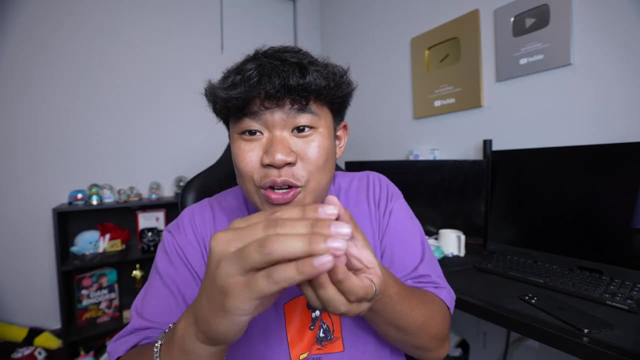 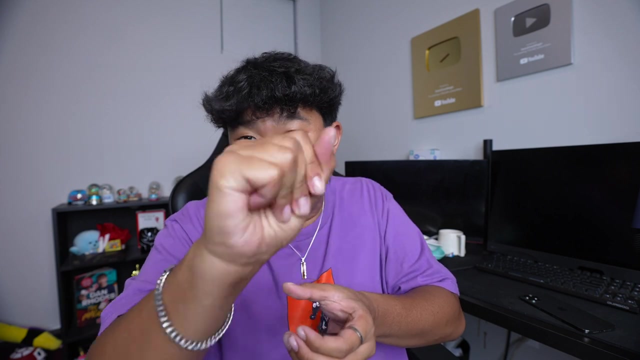 gonna let it drop. so once again, you want your thumb at the top, four fingers at the bottom. you're gonna use your other hand to cover the action, bring your thumb through that hole and as soon as you're covering the front view, as soon as the cap is covered, drop the cap, pretend to grab with the other hand. so 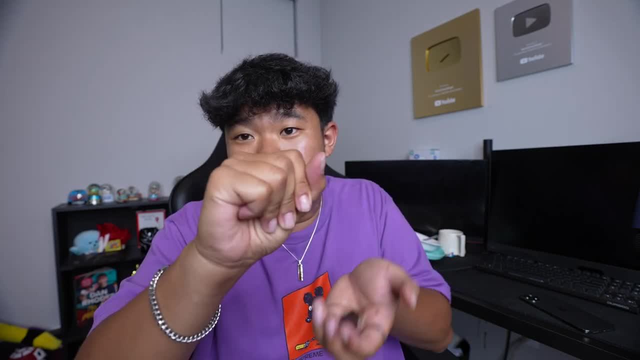 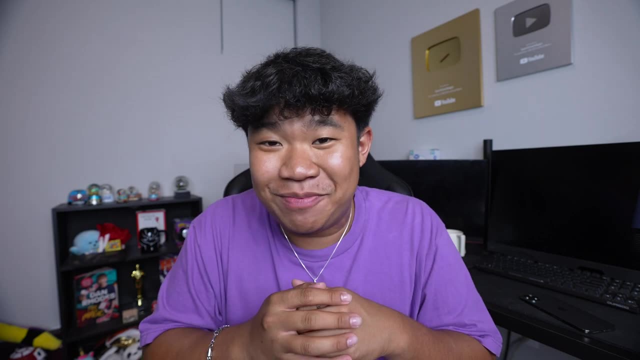 the focus will be on this hand and bring this other hand with the actual cap. bring this down. they're gonna think that the cap is in this hand. you're gonna blow, it vanishes and bam, you're an instant magician. all together, it should look something like this: 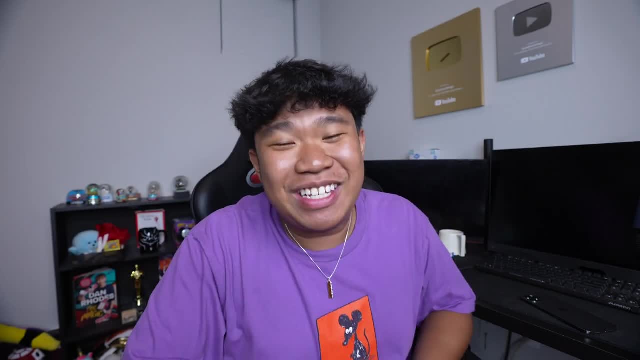 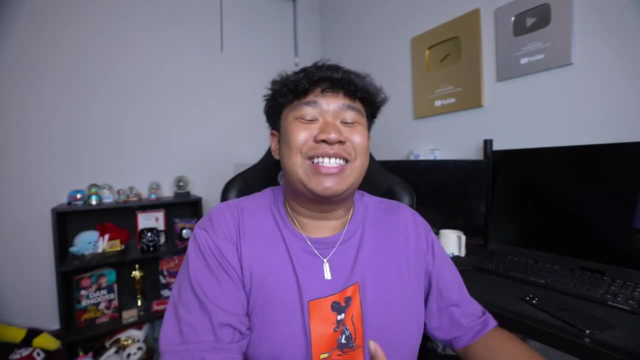 watch vanish. so yeah, those are five easy magic tricks that you can do at school right now. go get yourself some friends, because I never did. in all seriousness, if you enjoyed the video, make sure you like and subscribe more tutorials out soon and I'll catch y'all in the next one.